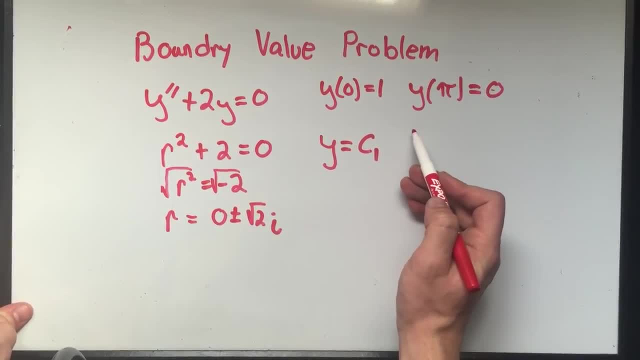 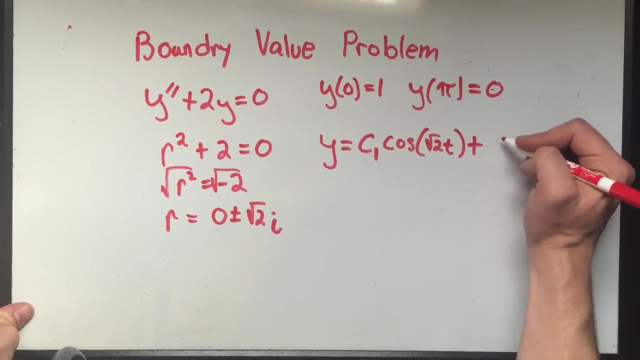 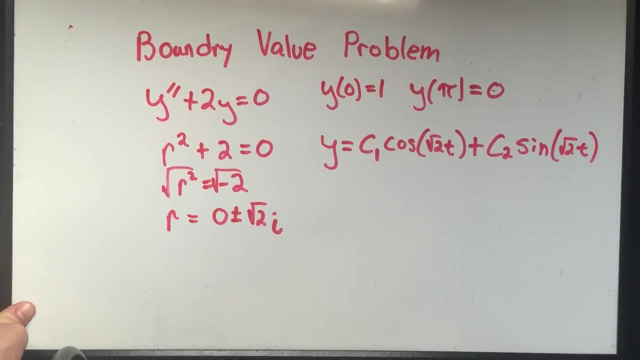 would be like C1, e to the 0.. I'm not gonna write e to the 0 because it's 1, but it'll be cosine of square root of 2t plus C2 sine square root of 2t. So if you've, 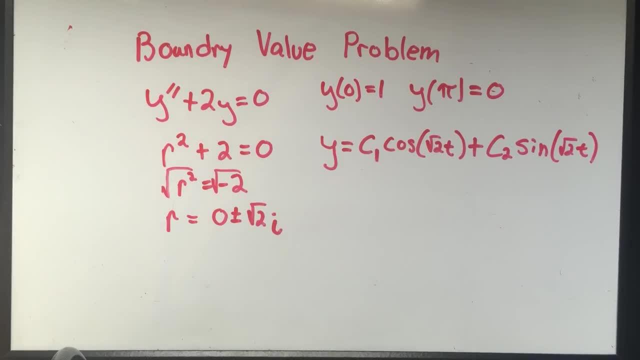 learned everything you need to learn about second-order differential equations. this comes as no surprise to you, And this is all just very, very similar, very straightforward. so now I'm just going to solve for my C1 or C2, right? This is my general solution. I want my specific solution. So if I plug, 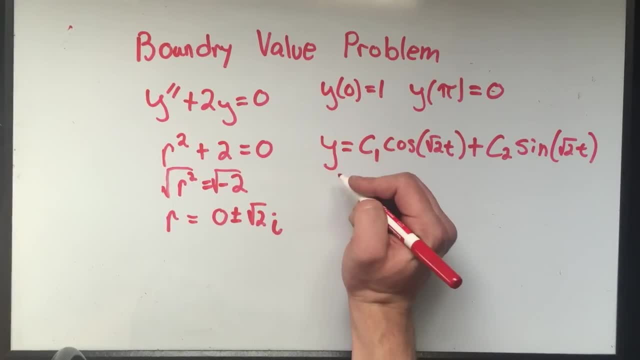 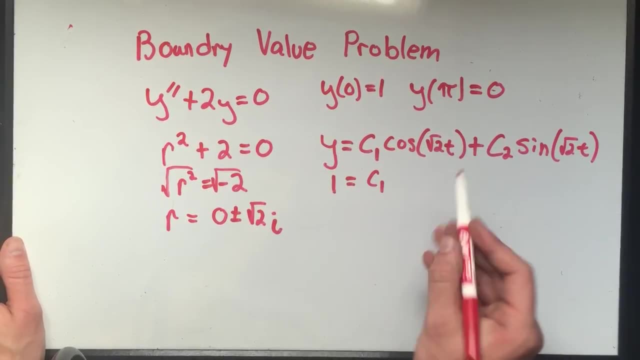 in 0 for t, I better get 1.. So this says that 1 has to equal C1 cosine of 0.. 0 is 1, plus well, sine of 0 is 0, so this would be plus 0.. 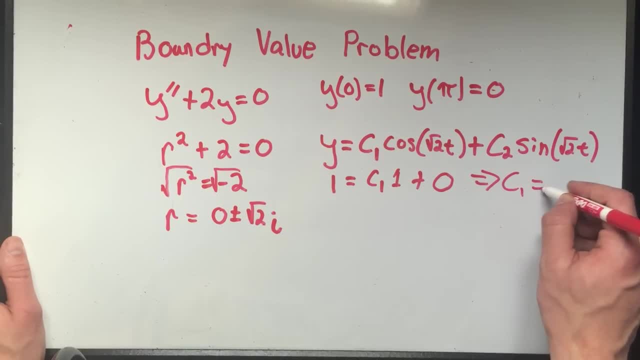 So it looks like C1 is 1.. Okay, and I also know that if I plug in pi I'm going to get 0. So let me make a second line here. I get 0 if I plug in pi and remember that we just found C1 to be 1, so I'm going to. 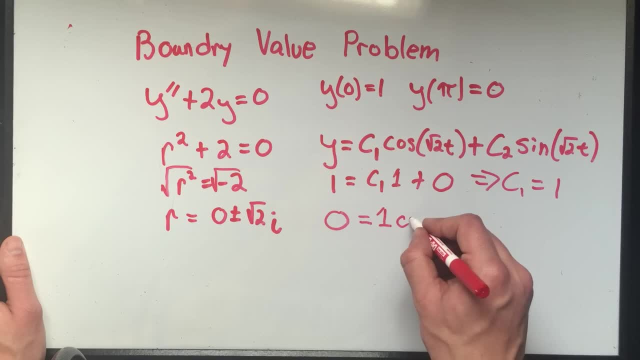 write that 1 cosine of square root of 2 pi plus C2 sine square root 2 pi. Okay, Now I can solve for C2, so I'm not even going to bother writing times 1.. If I subtract cosine, the minus cosine of square root 2 pi. sorry, this is an ugly number. 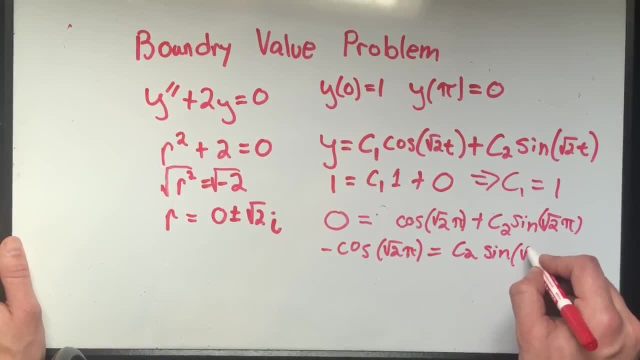 equals C2 sine square root 2 pi. Now if I divide both sides by sine, I get a minus cosine square root 2 pi over a sine squared root 2 pi. Hey, would you look at that? cosine over sine, that's cotangent square root 2 pi.